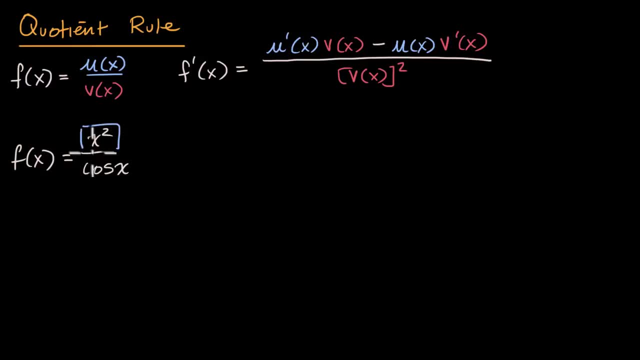 and what could be our v of x? Well, our u of x could be our x squared. So that is u of x, and u prime of x would be equal to two x. And then this could be our v of x. So this is v of x. 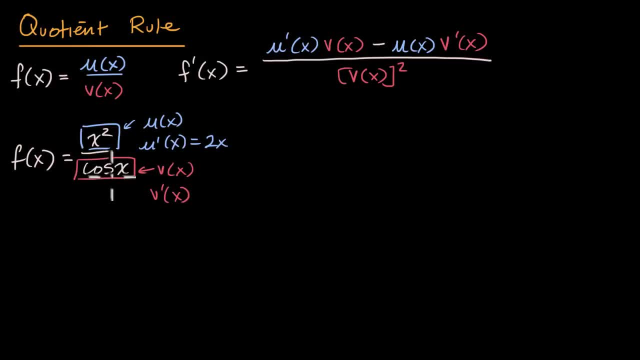 and v prime of x, the derivative of cosine of x with respect to x is equal to negative sine of x, And then we just apply this. So, based on that, f prime of x is going to be equal to the derivative of the numerator function. 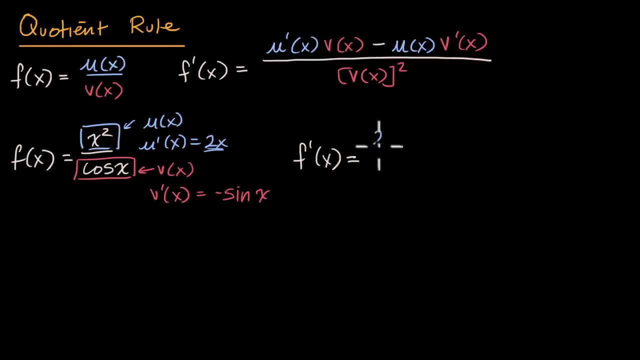 That's two x right over here. That's that there. So it's gonna be two x times the denominator function. V of x is just cosine of x times cosine of x. V of x is just cosine of x times cosine of x. 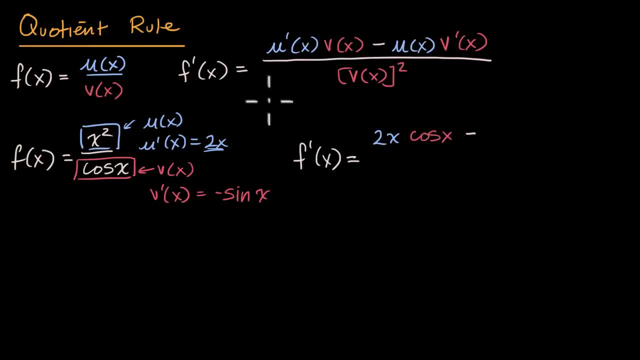 V of x is just cosine of x times cosine of x, Minus the numerator function, which is just x squared x squared times the derivative of the denominator function. The derivative of cosine of x is negative sine x, So negative sine of x. 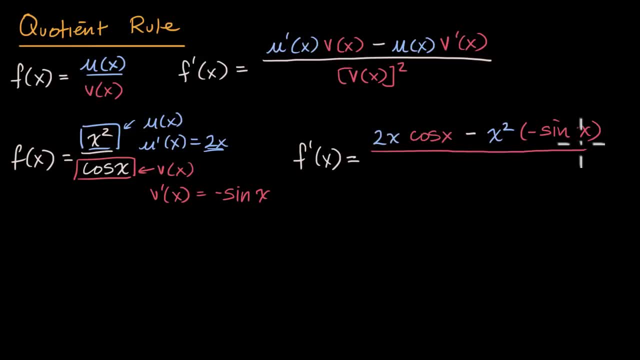 All of that, over all of that, over the denominator function squared. So that's cosine of x, and I'm going to square it. I could write it, of course, like this: Actually, let me write it like that, just to make it a little bit clearer. 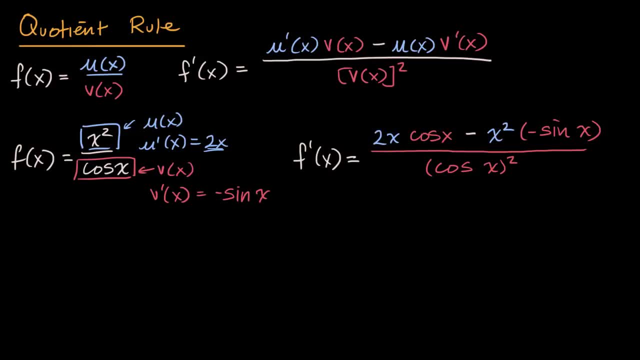 And at this point we just have to simplify. This is going to be equal to: let's see, we're gonna get two x times cosine of x, Two x cosine of x. Negative times a negative is a positive Plus x squared x. squared times sine of x. 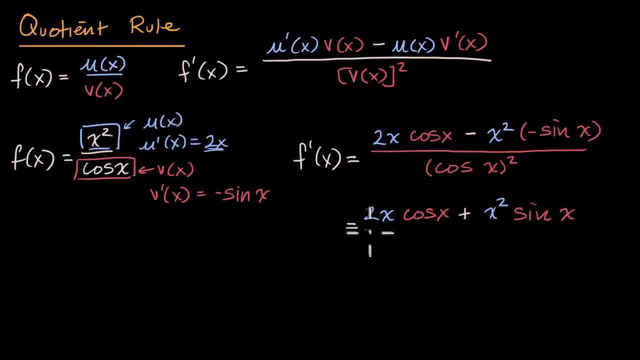 Sine of x, All of that over Cosine of x squared, which I could write like this as well, And we're done. You could try to simplify it. In fact, there's not obvious ways to simplify this any further. 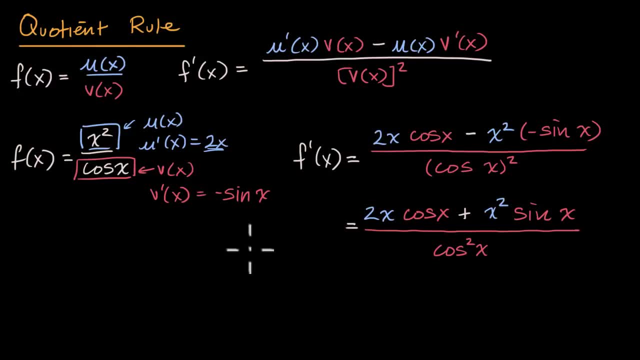 Now what you'll see in the future. you might already know something called the chain rule, or you might learn in the future, But you could also do the quotient rule using the product and the chain rules, which you might learn in the future. 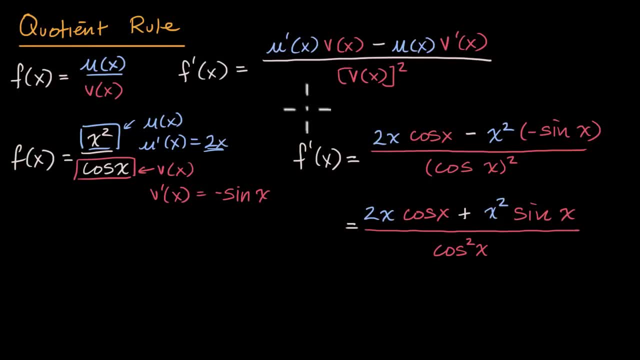 But if you don't know the chain rule yet, this is fairly useful.